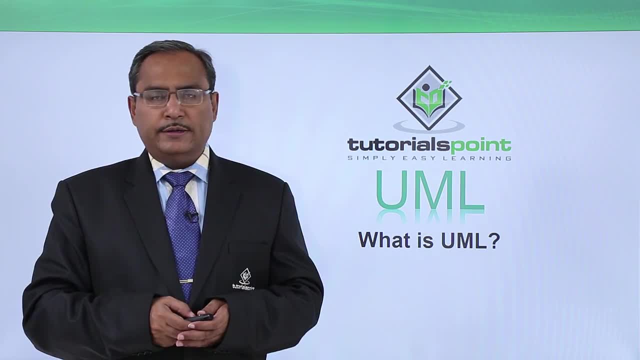 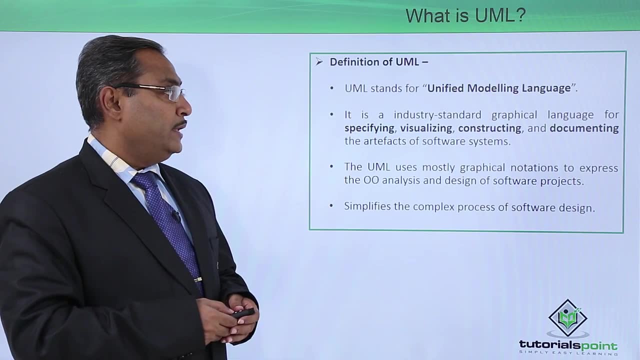 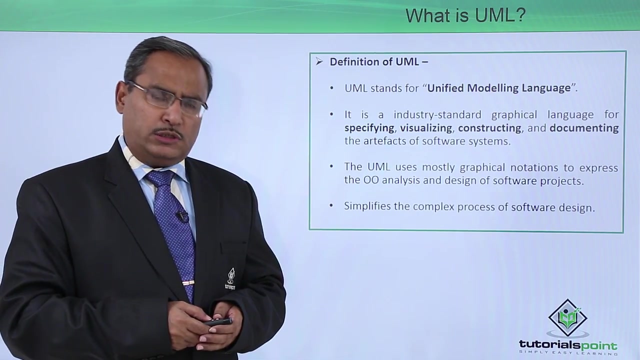 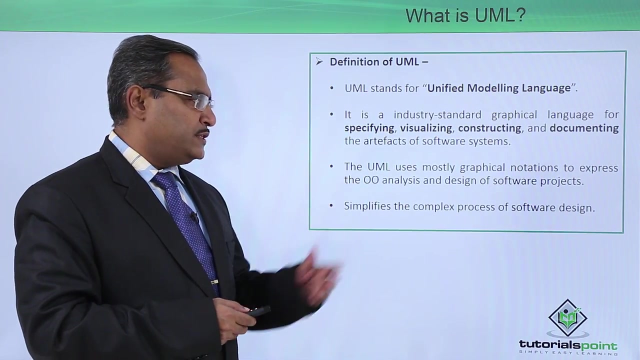 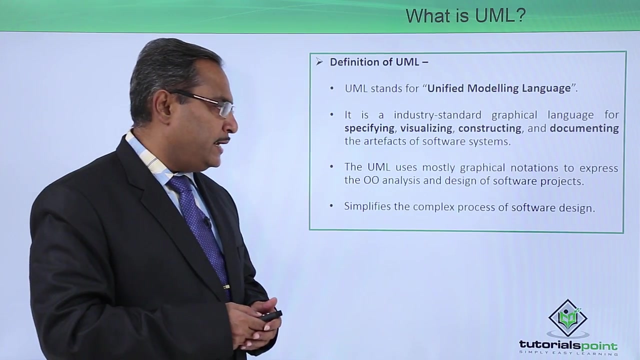 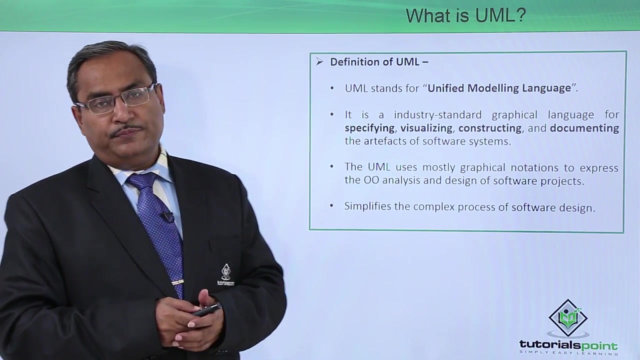 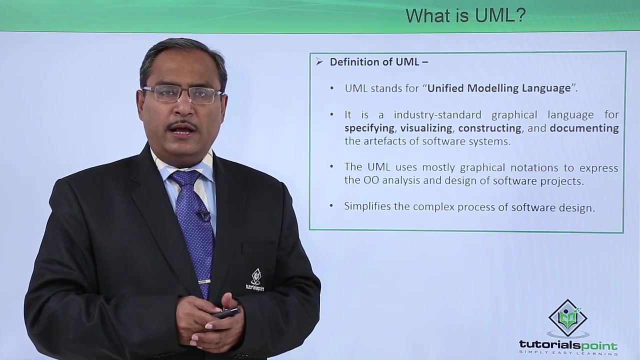 What is UML? So we are going to define UML. UML stands for Unified Modeling Language. It is an industry standard graphical language for specifying, visualizing, constructing and documenting the artifacts of software system. The UML uses mostly the graphical notations to express the object oriented analysis and object oriented design of software projects and simplifies the complex process of software design. So UML is having the full form, that is, the unified modeling language, with the help of which we are going to have some graphical representations, some pictorial representations of a software system. 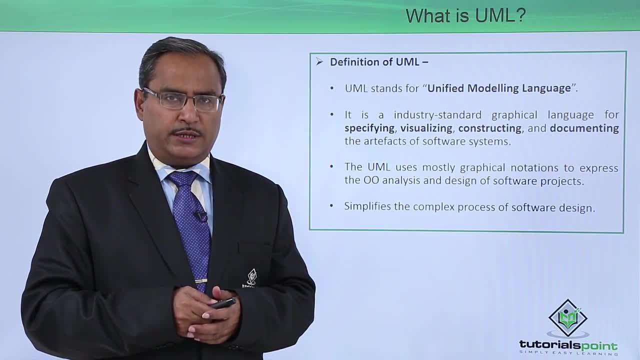 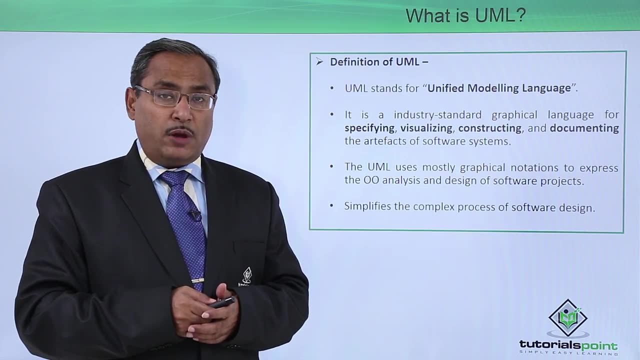 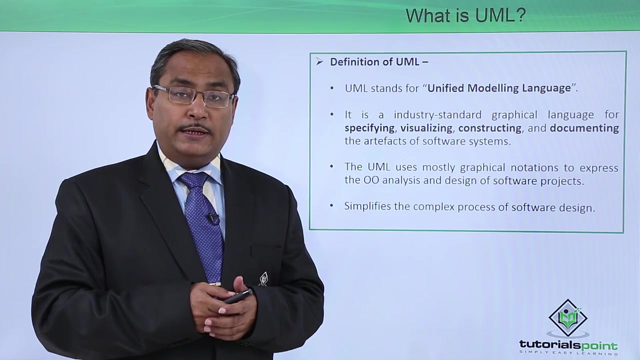 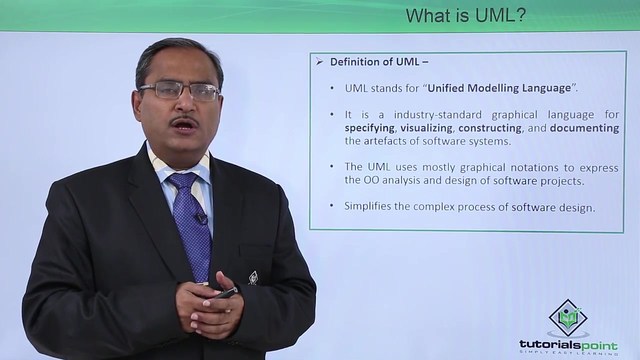 So before getting into the UML, let us take a look at the UML. So before getting into the UML, let us take a look at the UML. Before getting a software implemented, before getting the software tested, we should gather all the requirements from the client. And all these requirements, if you can put them in some proper graphical and pictorial representation, then that will be quite easy for the people who are working within the project or stakeholders of the project to communicate in between each other. So that's why it is a very popular tool for the graphical representation of the UML. 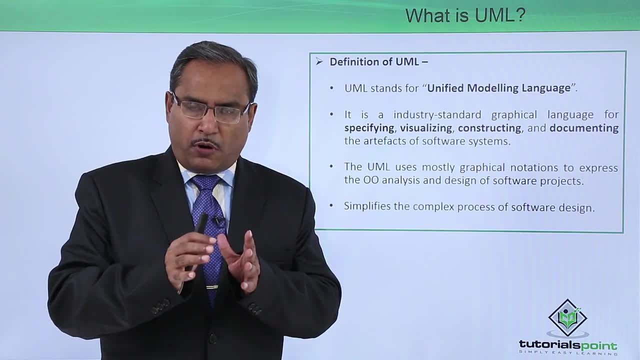 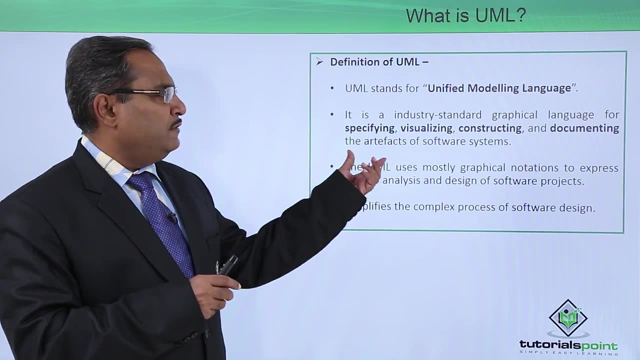 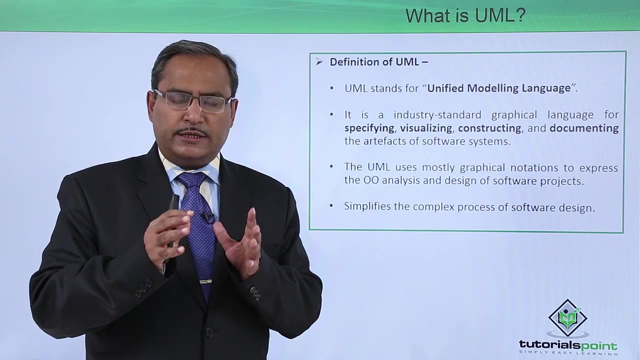 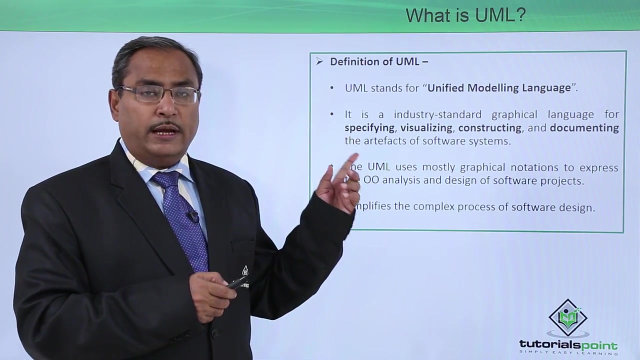 Before getting a software implemented. before getting a software implemented, before getting a software implemented, we should gather all the requirements from the client And all these requirements, if you can put them in some proper graphical representation, then that will be quite easy for the people who are working within the project or stakeholders of the project to communicate in between each other. 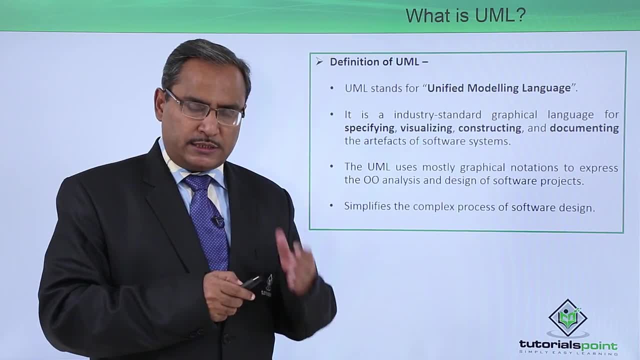 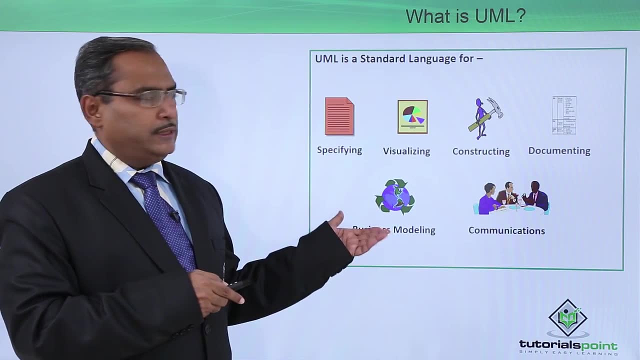 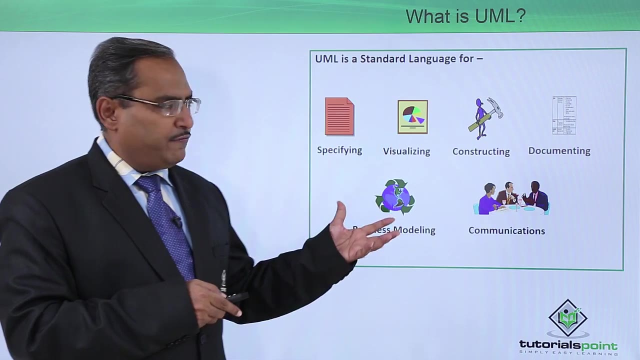 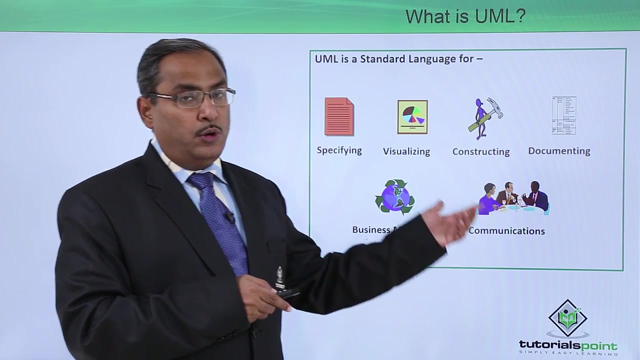 Before getting a software implemented. before getting a software implemented, before getting a software implemented, we should gather all the requirements from the client And all these requirements, if you can put them in some proper graphical representation, then that will be quite easy for the people who are working within the project or stakeholders of the project to communicate in between each other. 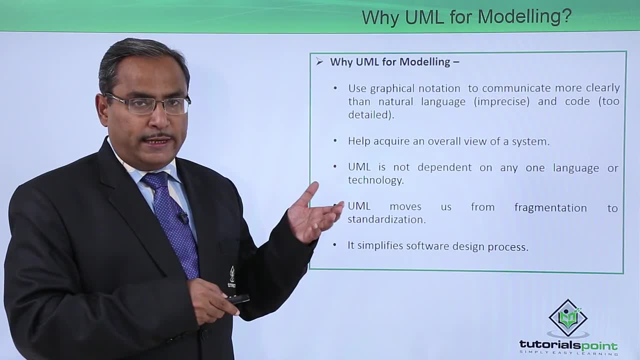 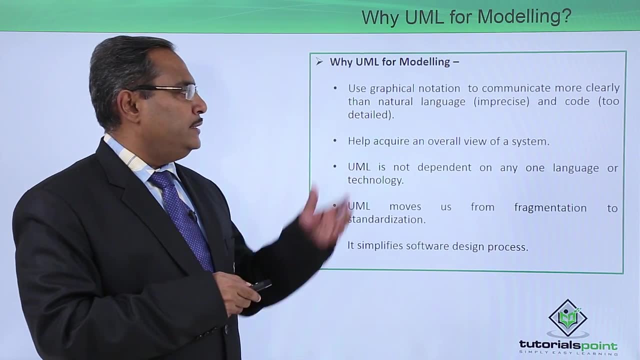 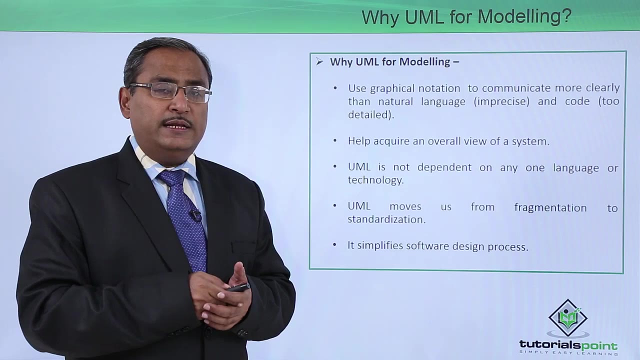 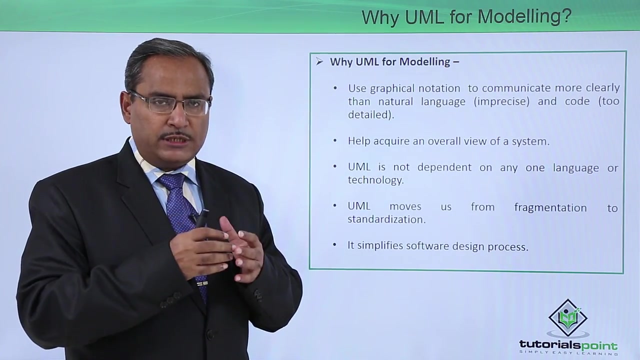 Before getting a software implemented. before getting a software implemented, before getting a software implemented, we should gather all the requirements from the client And all these requirements, if you can put them in some proper graphical representation, then that will be quite easy for the people who are working within the project or stakeholders of the project to communicate in between each other. 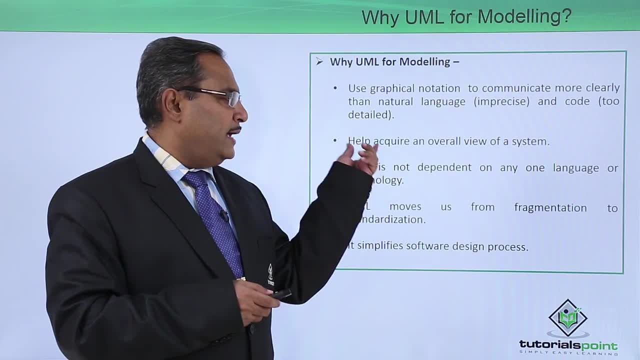 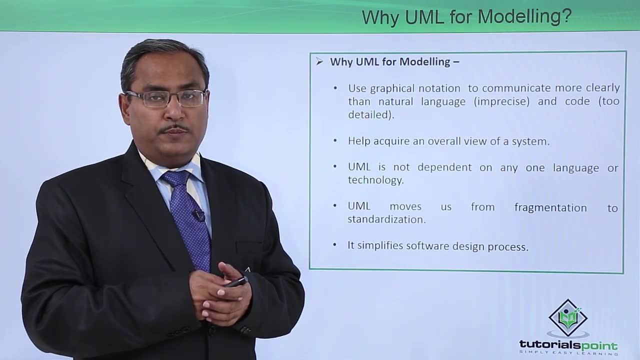 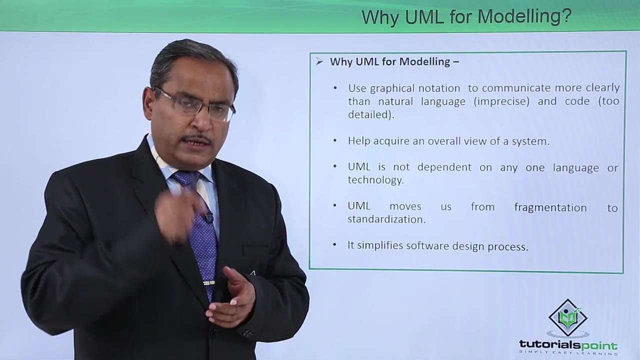 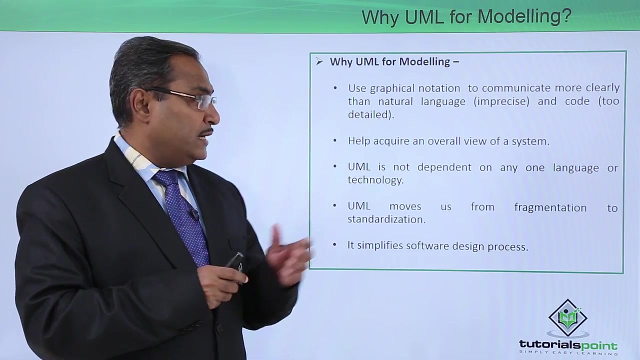 Before getting a software implemented. before getting a software implemented, before getting a software implemented, we should gather all the requirements from the client And all these requirements, if you can put them in some proper graphical representation, then that will be quite easy for the people who are working within the project or stakeholders of the project to communicate in between each other. 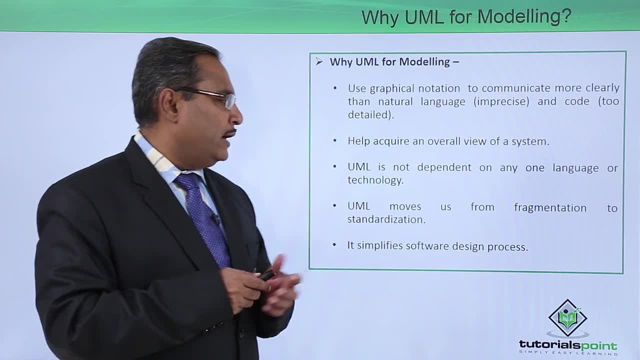 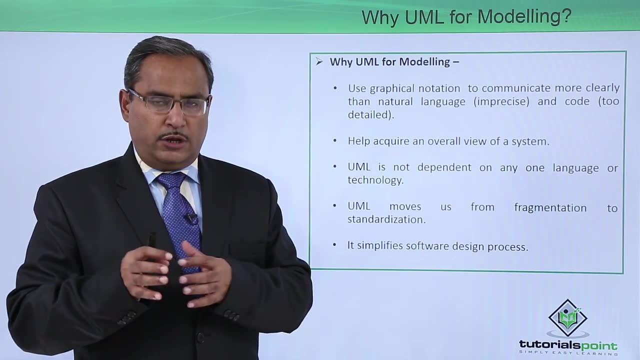 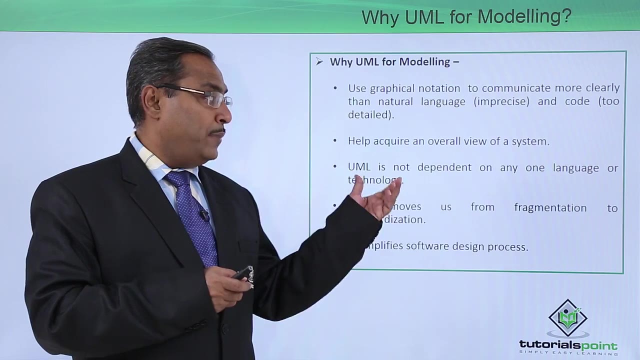 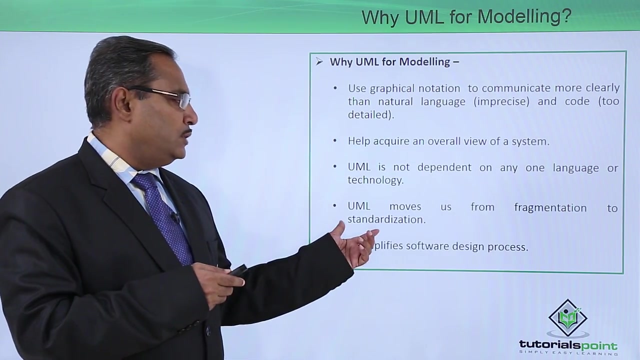 Before getting a software implemented. before getting a software implemented, before getting a software implemented, we should gather all the requirements from the client And all these requirements, if you can put them in some proper graphical representation, then that will be quite easy for the people who are working within the project or stakeholders of the project to communicate in between each other. 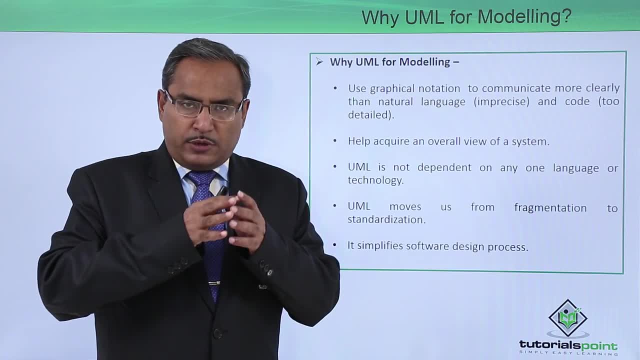 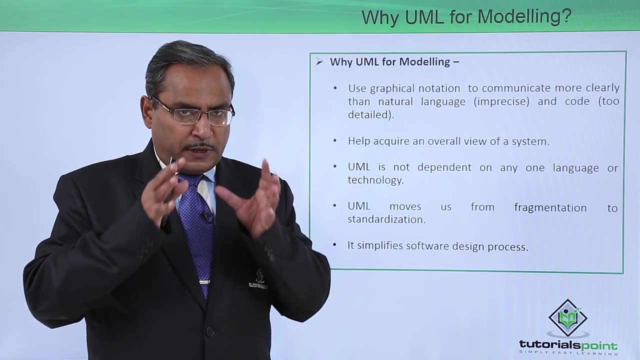 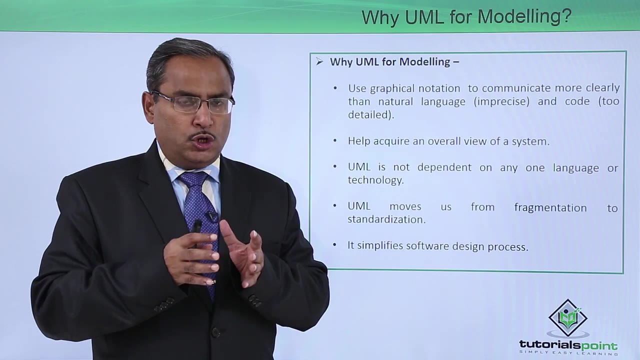 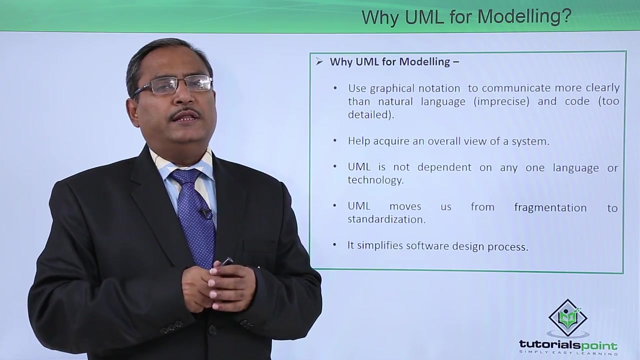 Before getting a software implemented. before getting a software implemented, before getting a software implemented, we should gather all the requirements from the client And all these requirements, if you can put them in some proper graphical representation, then that will be quite easy for the people who are working within the project or stakeholders of the project to communicate in between each other. 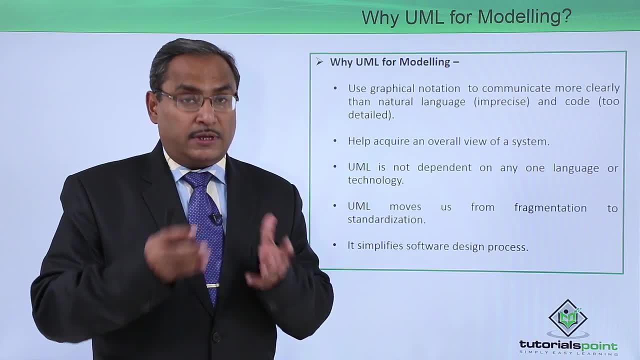 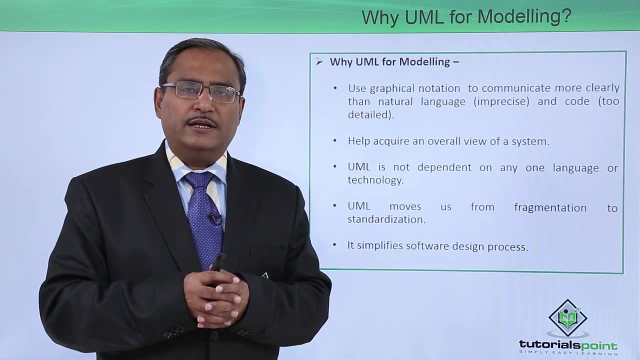 Before getting a software implemented. before getting a software implemented, before getting a software implemented, we should gather all the requirements from the client And all these requirements, if you can put them in some proper graphical representation, then that will be quite easy for the people who are working within the project or stakeholders of the project to communicate in between each other.